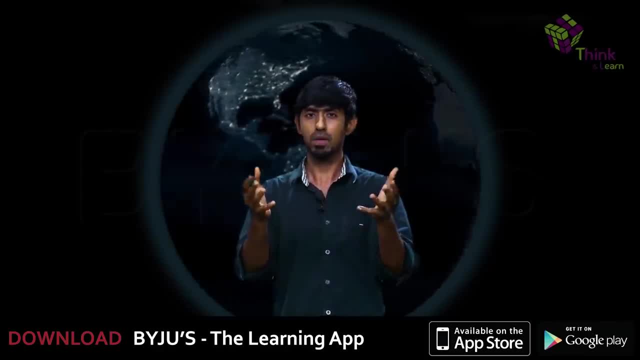 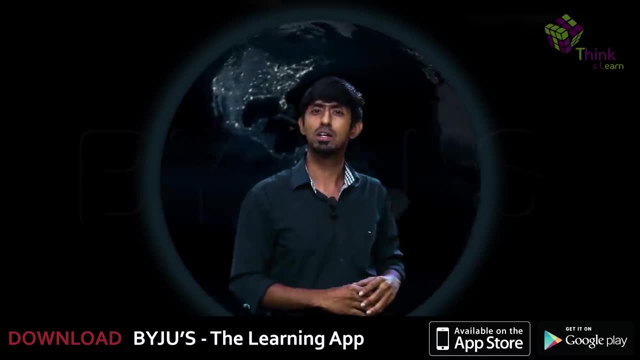 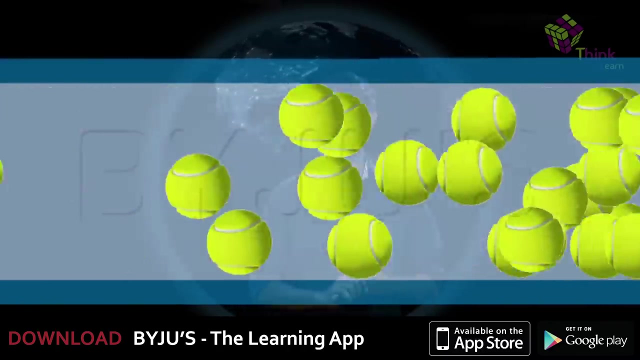 Now the question then for us is what we mean by current. for our purpose, here is simply a large number of some kind of balls moving in some general direction, as they're banging against each other. So it's time to test yourself. If I ask you now, if you know the current is in that direction- let's say a tennis ball current- then can you say that every single tennis ball, at every single point in time, is going in that direction? 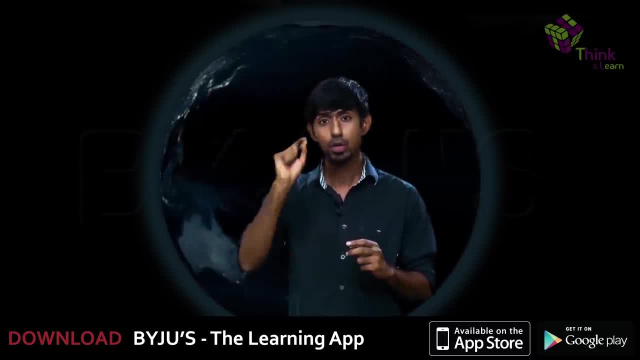 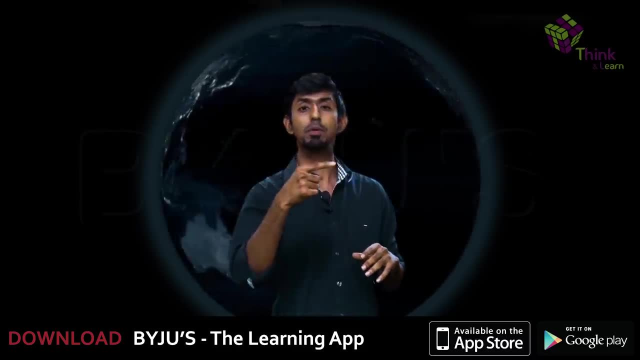 Can you even say that a tennis ball at some point should have gone in that direction? Think about it. Yes, The thing to notice here is, even though the current might be in that direction, each of the individual balls might be going in some random direction. 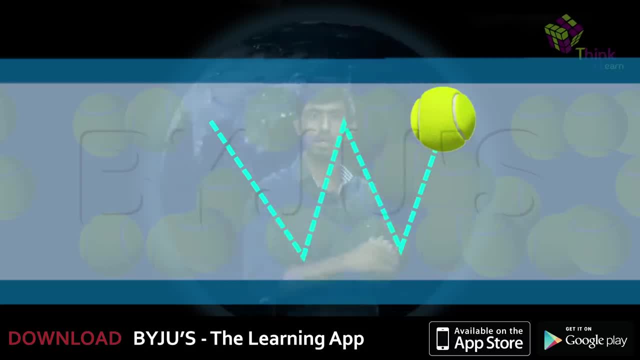 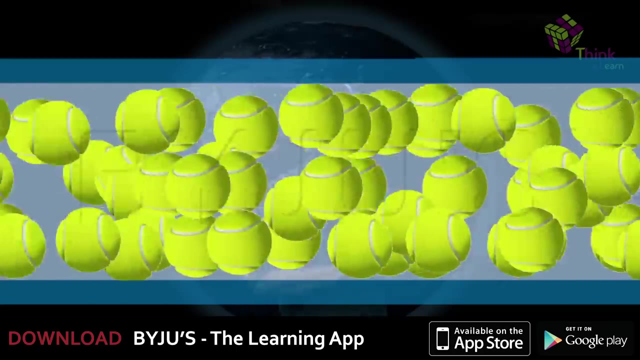 In fact, if you pick one ball, it might be doing something like this, A zigzag motion, such that at no point it is actually ever pointing exactly in the direction of the current. So it is possible. So if you thought that the balls must also go in the direction of the current, you might have imagined the pipe to be containing balls that are beautifully parading like that. 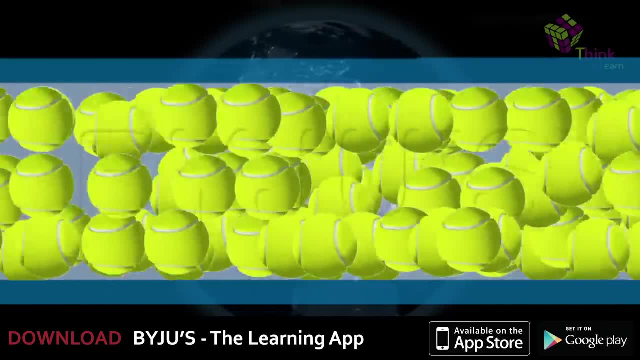 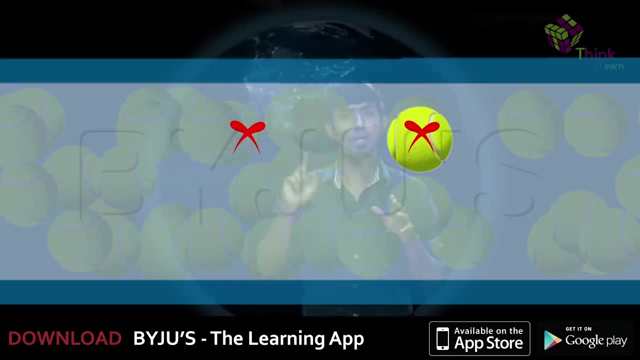 But in reality you know that all we're saying when we say there's a current is that if you find a ball here, if you mark it and then you look after some time it will be somewhere over there. We are not telling anything about the actual path it's taking. It takes some random path like that. 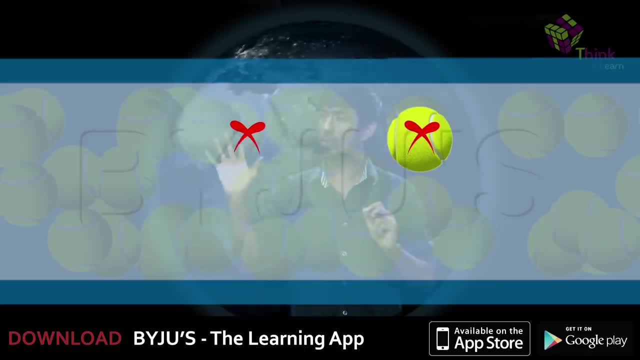 Never be exactly in the direction of the current, But if at some time you see it here, after some time you can be sure it will be somewhere in that direction. That's what we mean when we say there is a current in that direction. 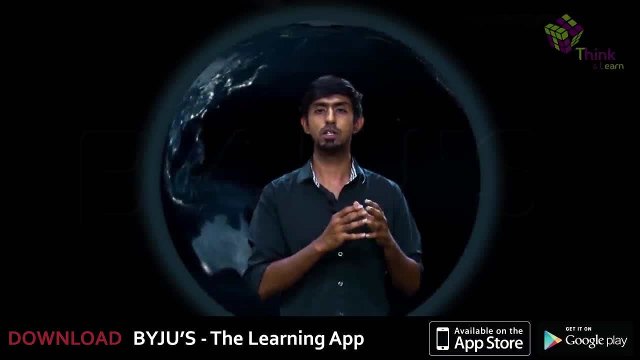 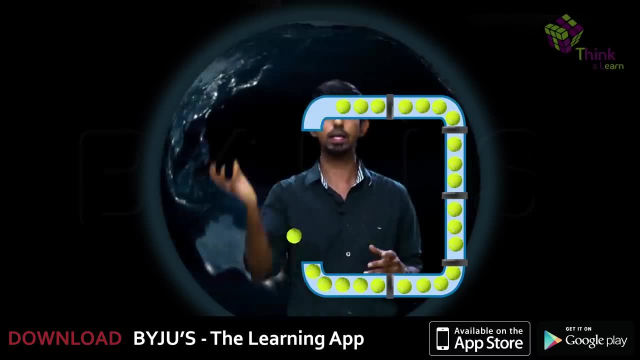 Now, if I want to set up a current of tennis balls in a pipe that looks like a C, like this, Then I can collect one from below. that will create a small gap. I push it back from the top And I can keep doing this. 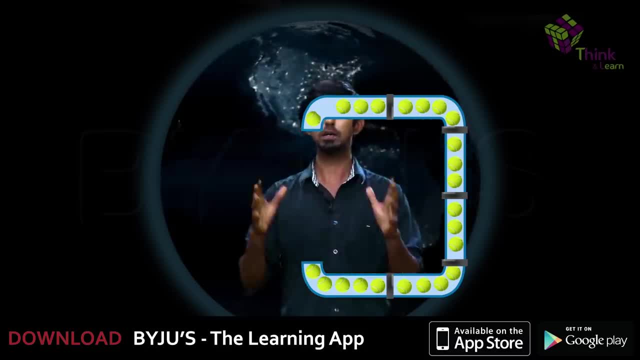 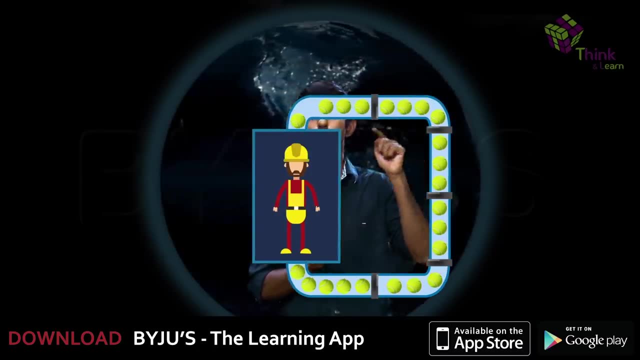 And after a while I'll get really bored. I can hire somebody to do it. Let me hire a man who is trapped in a box Which has only two holes, One below and one on top, So I connect the two ends of this pipe to those holes. 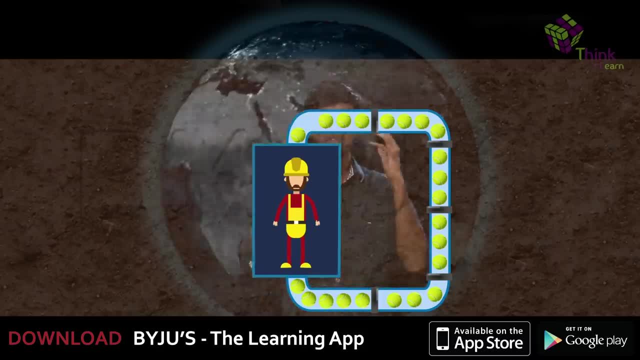 And I bury this whole thing underground. You're thinking: what are we even doing And why are we burying this person underground? We'll talk about that. You'll understand why we're doing this, But for now, here's a man buried underground with only two holes. 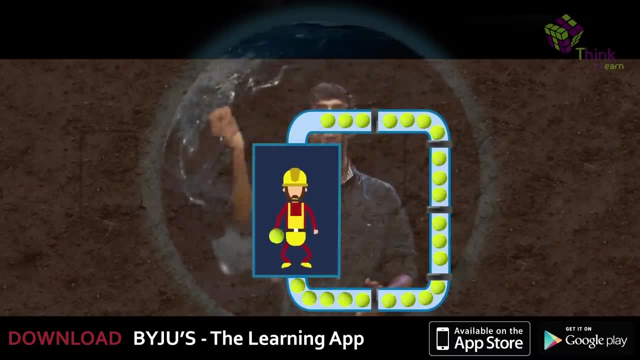 Right And he keeps picking up balls from the bottom part and puts it on the top, again Below, And he keeps doing this all the time, Thereby maintaining this current of tennis balls into the box, Into the box and out of it. 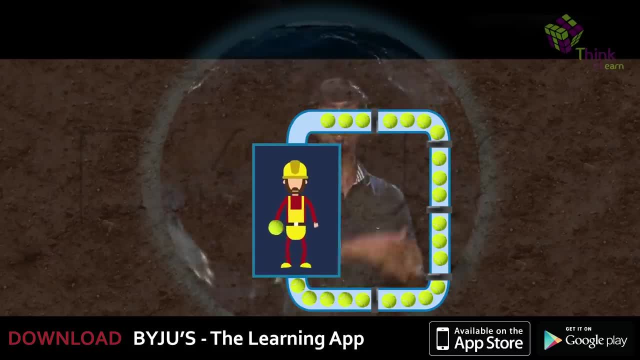 Now, this man is very hardworking. okay, He keeps picking up the ball, keeping it on top, thereby maintaining the current. But what if he gets tired and stops doing what he's doing? What will happen to the current of tennis balls? 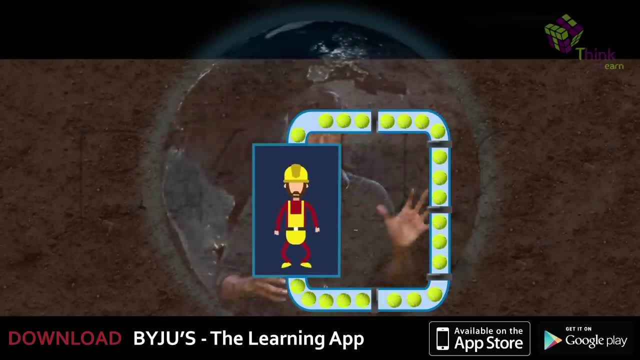 So if you watch what's happening, he's pulling a ball out, creating a gap, Which is creating a gap on top, And then he pushes the ball back in over there. Now, if he stops doing this after this, there's no gap created. 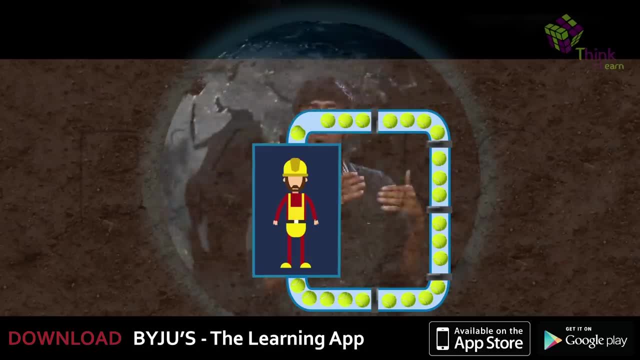 There's nothing for anything to move, So all the balls are going to remain stationary. In other words, the current has stopped. Now let's take this man and put him under slightly different work conditions. Let's tell him: listen, the pipe is gone. 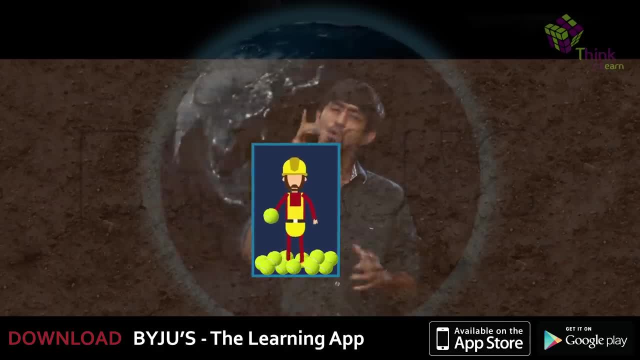 Now there are some few balls below you. You carry them and do what you were doing before: only Carry one up and keep it up, but hold them there So that you're continuously doing this. After a while, he is holding a few balls on top. 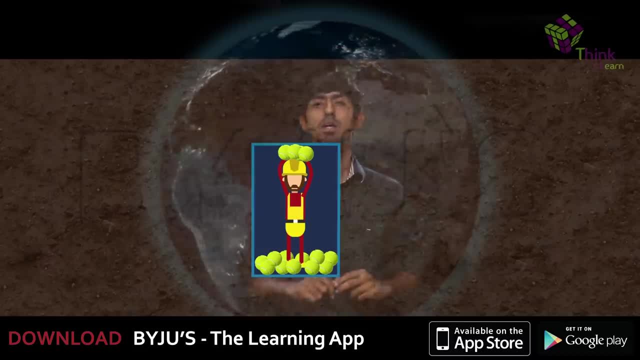 Right, He has to do some work to do that. Right, He's holding them there And he's done some work to take them there. Now, this picture of a man holding balls up waiting for a pipe to someday come So that he can begin his current. 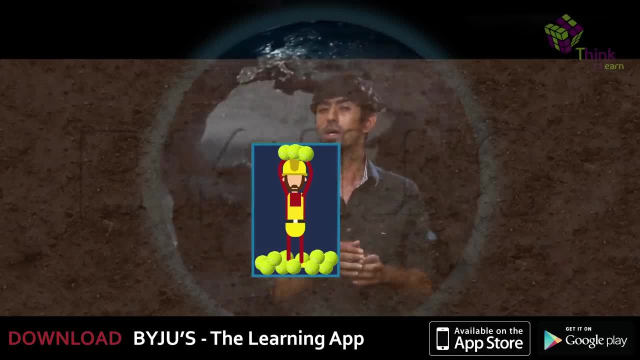 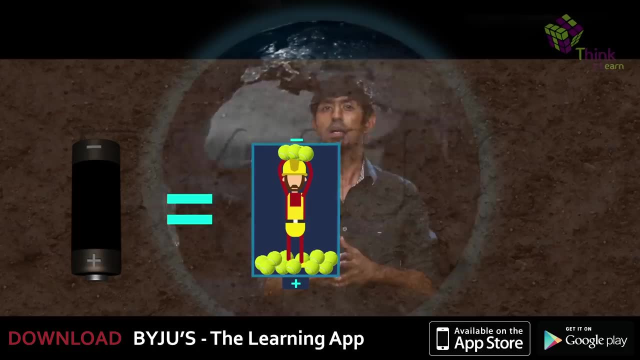 After which he can start doing his old job, Is our cell. Because now, if we draw out what looks like a typical cell around this And if we name the man inside Chemical X, Now something chemical is happening. We can't tell you more right now. 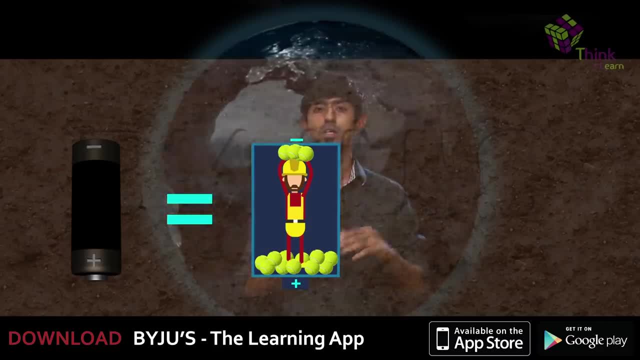 And then if we tell you, instead of holding up tennis balls, This whole thing over there, Those balls that he's holding up are smaller than even water balls, Smaller than even air balls. They are balls that are extra small, Extremely small. 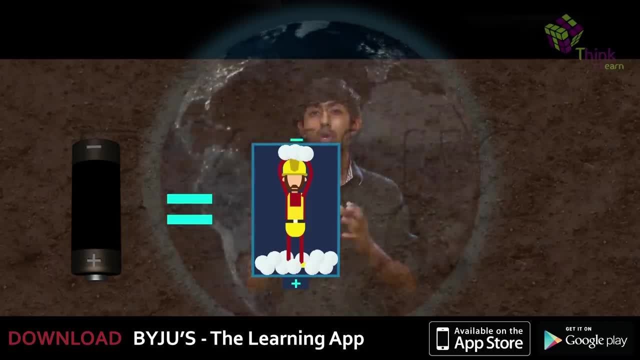 Probably the smallest balls we know, Called electrons. Now, what these electrons are and all that and all we'll learn later. Okay, Then what if I tell you everything now, What you do in 7th, 8th, 9th, 10th and all? 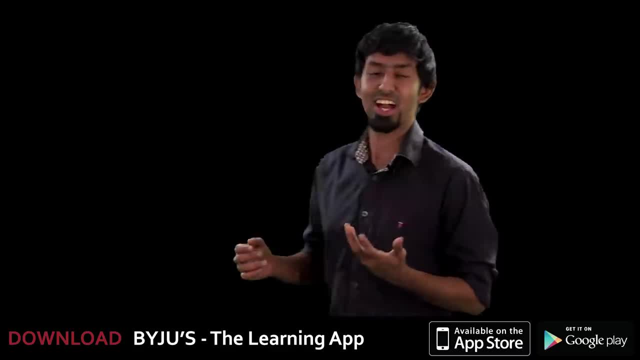 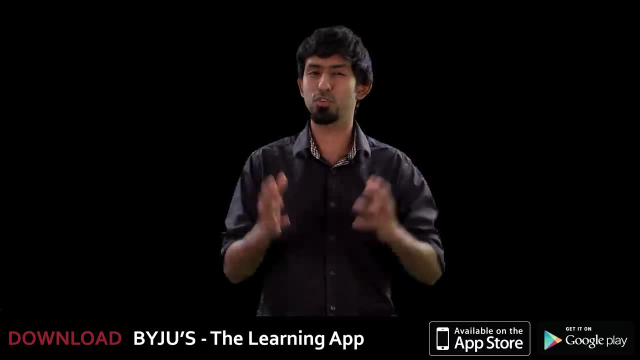 So that we'll learn later. So that was like a few minutes Right, And you already learned so much. If you want to learn much more, download the Byju's learning app. We made hours and hours and hours of content just for you to learn. Hope to see you there.